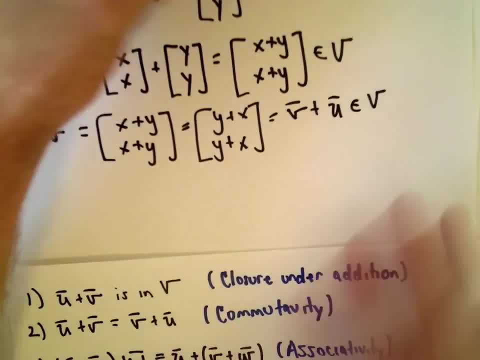 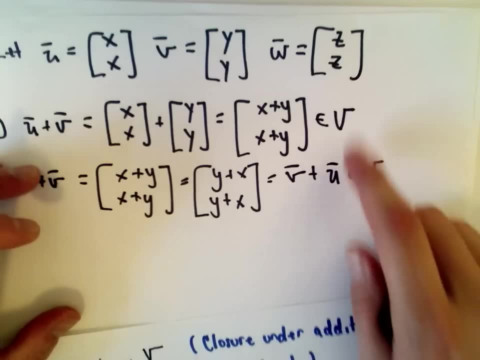 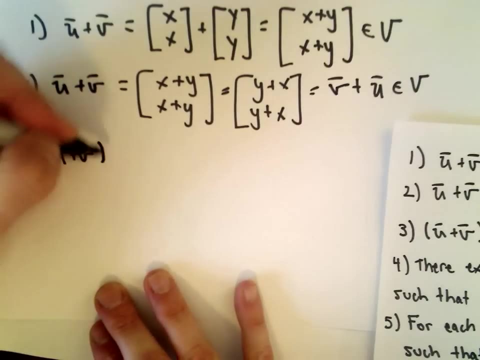 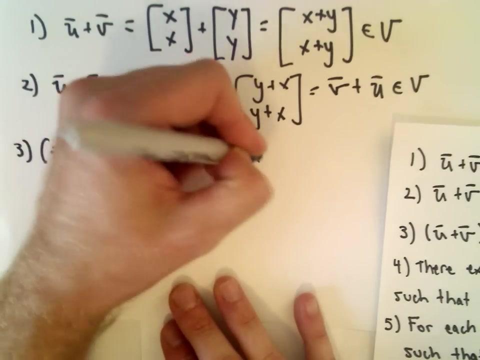 Well, no, come on, let's do it. So let's let vector w be a vector with components z and z. So let's see, We want to show that u plus v. if we do that first and then add w, is that the same thing as if we do u and then add v and w? 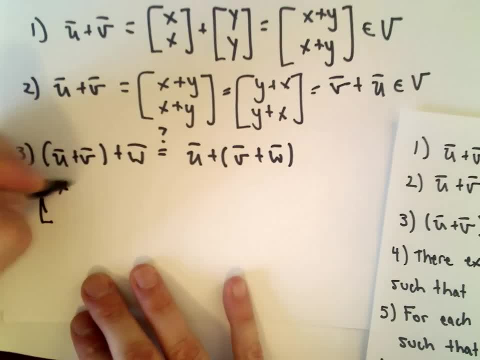 Well, u plus v. we said that's going to be x plus y Plus w. that would be. Now we have to add this extra vector. Well, that's going to give us x plus y plus z. x plus y plus z. 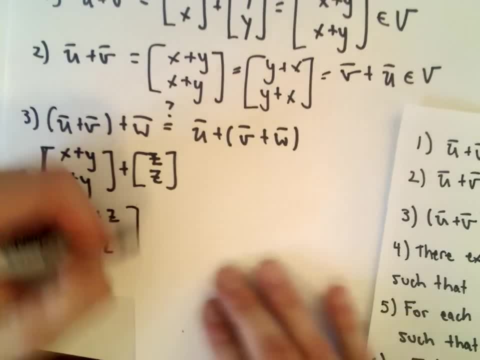 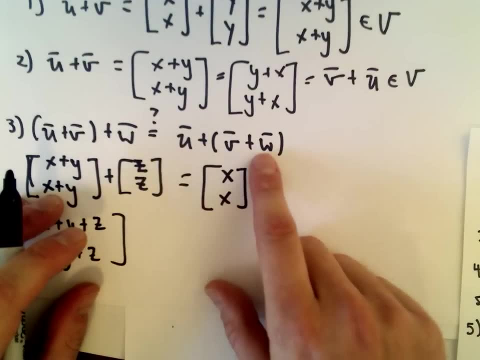 I think it's easy to see that you get the same thing on the other side. So if we do vector v plus w, we would have y plus z, y plus z, And if we do vector v plus w, we would have y plus z, y plus z. 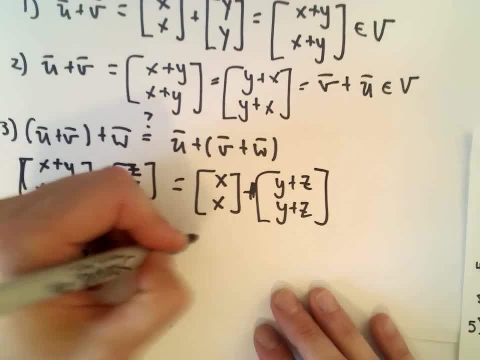 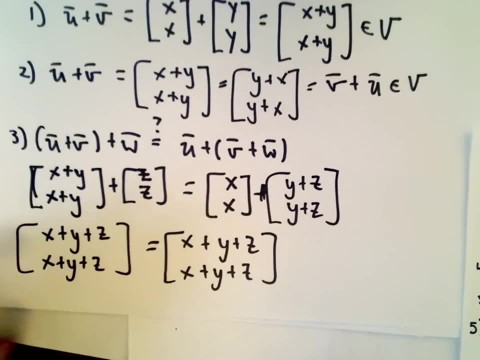 And if we do vector v plus w, we would have y plus z, y plus z, And if we add those together we'll have x plus y plus z, and we'll have x plus y plus z. So yeah, we get the same thing. 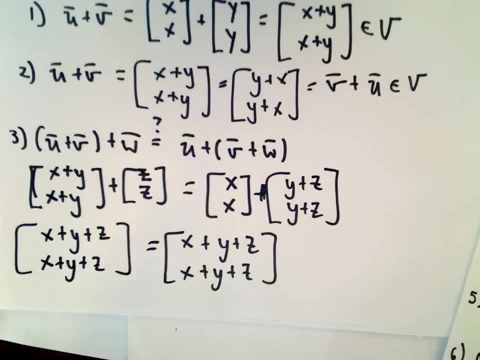 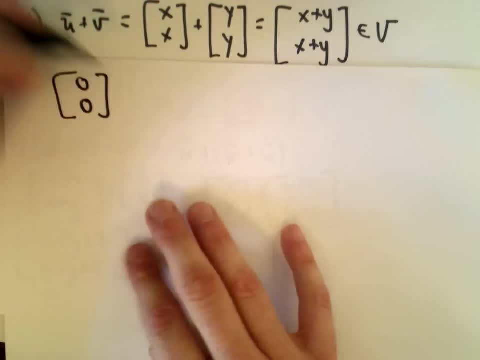 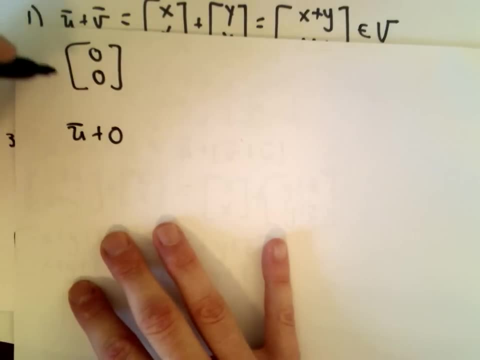 So it's definitely associative. Does there exist a zero vector? Well, yeah, the zero vector. So certainly zero. zero, that's in our set of vectors that were under discussion, And if we do So, the question is: does u plus zero? 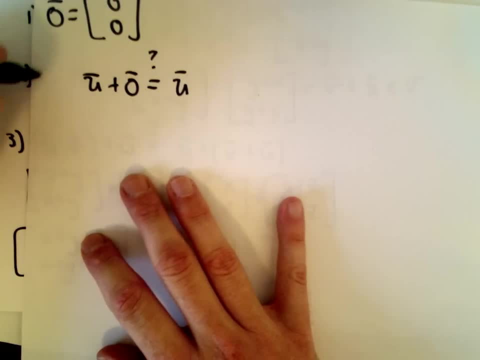 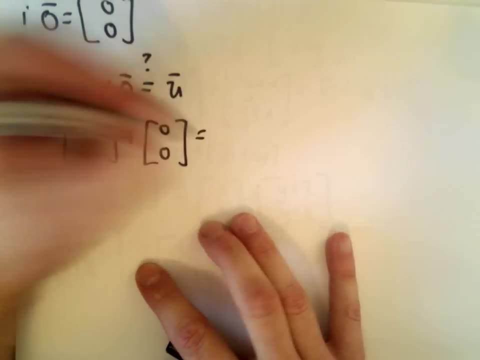 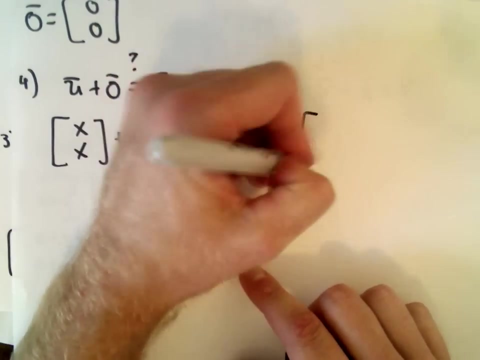 Does that equal u? So this will be property number four. Yeah, because then we have xx plus zero zero And again, if we add those, component-wise we'll get x plus zero, x plus zero, which is just xx. 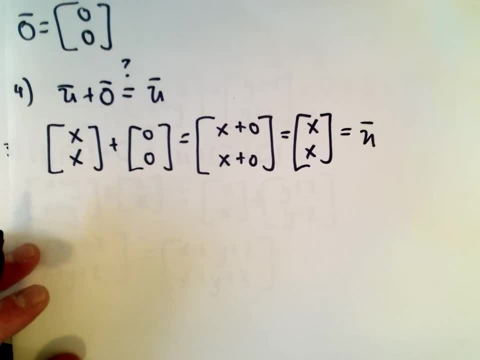 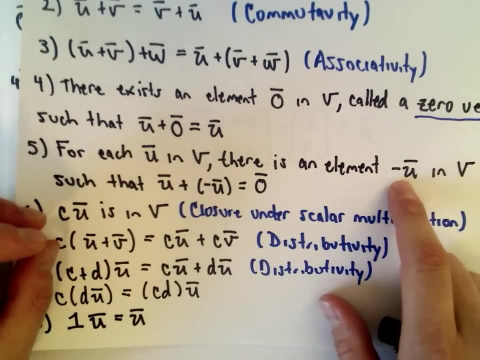 which is going to be our original vector that we started with. So okay, So for every vector in our space is there an element denoted negative of that in v, so that when we add them together we get the zero vector. 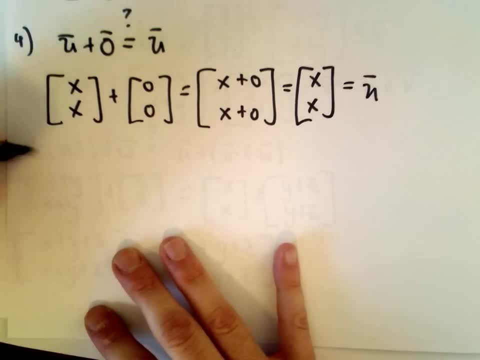 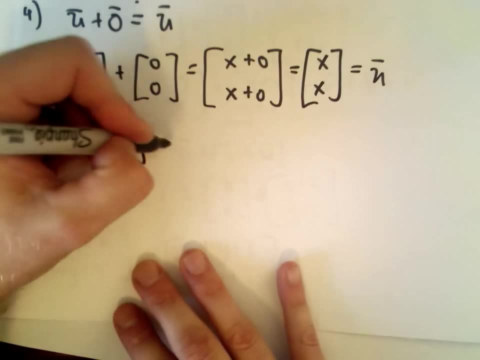 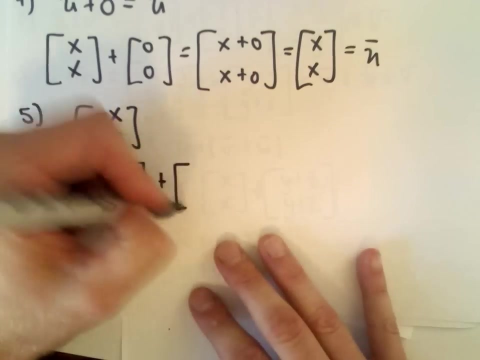 Sure, You know, if xx is in there, notice negative x, negative x. That's also of the form that we want, And if we take xx plus negative x, negative x, we'll just add those component-wise and get the zero vector. 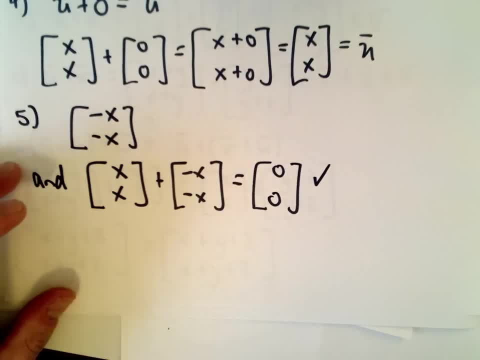 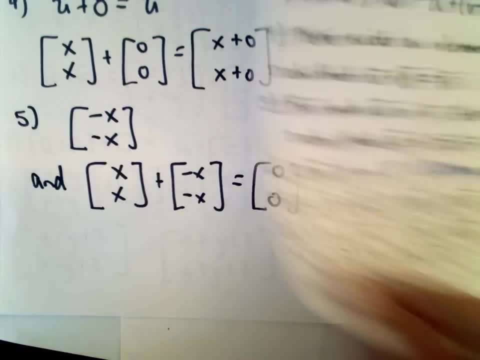 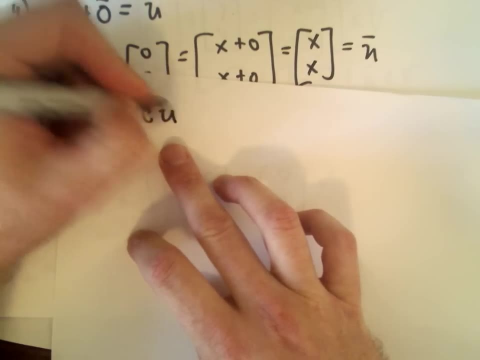 So no problem there either. There's definitely the negative of every element. Let's see: If we take c and multiply it by u, is that in v? Well, definitely So. property number seven. So if we take c and multiply it by u, 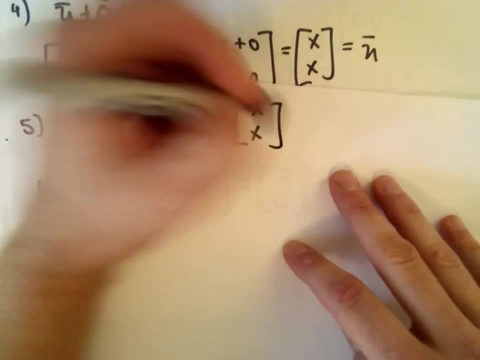 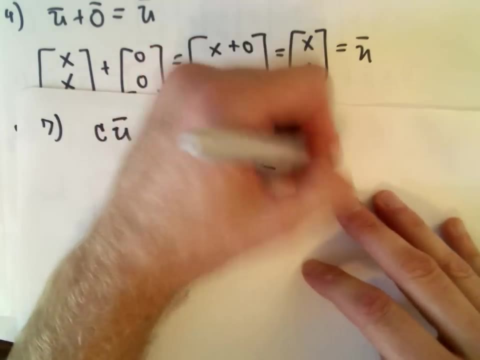 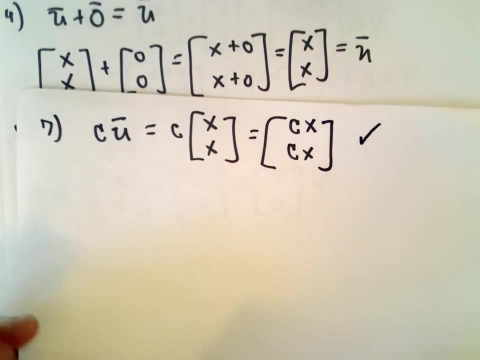 well, that's going to be c multiplied by the vector with components xx. We just multiply each component by c, And again, when we do that scalar multiplication, we do in fact get a vector that has the same components. So no problem there. 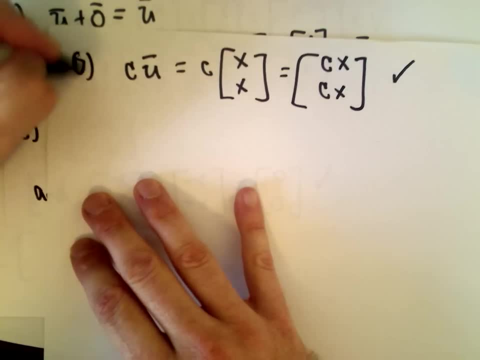 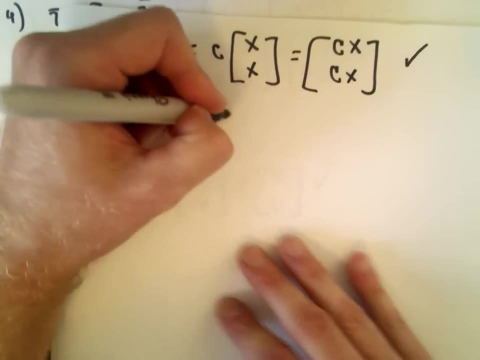 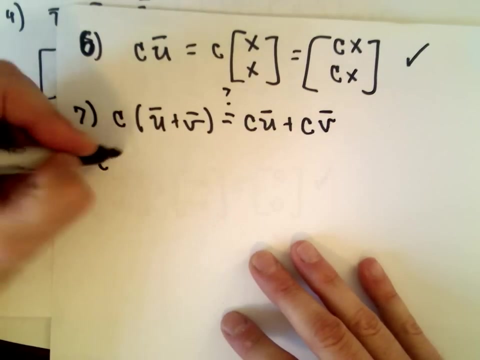 Let's see. That's actually property number six, Property seven: We have to show that c multiplied by the quantity u plus v Does that equal c multiplied by u plus c multiplied by v? Well, let's see, We've already seen that u plus v would be x plus v. 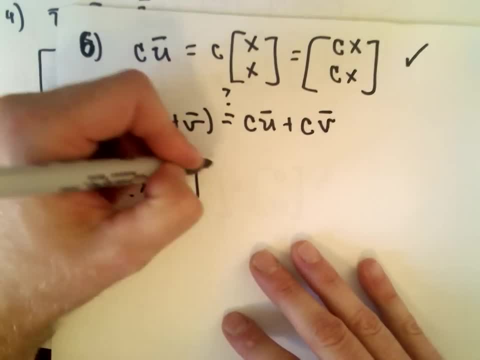 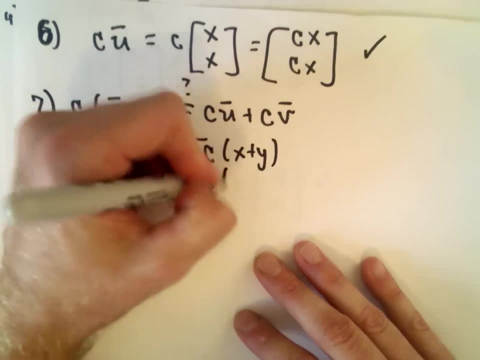 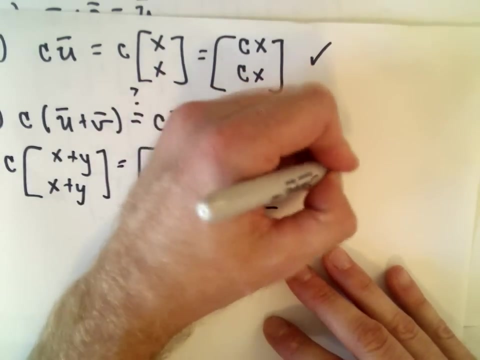 v would be x plus y, x plus y. So if we distribute, we would have c multiplied by x plus y, c multiplied by x plus y. Well, if we distribute, we'll have cx plus cy, cx plus cy. 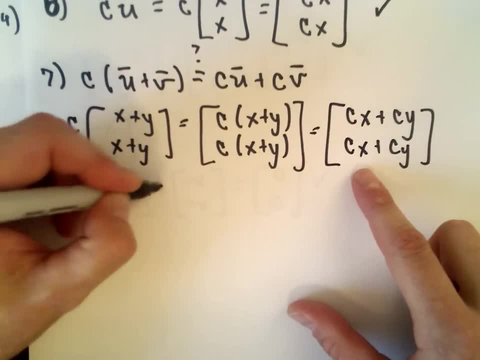 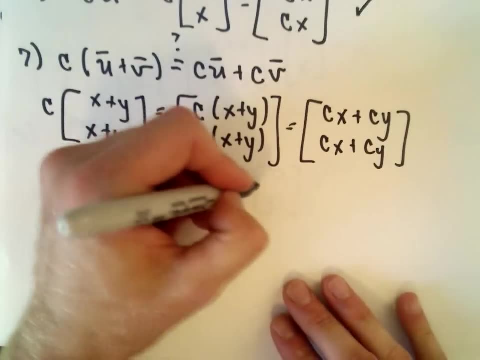 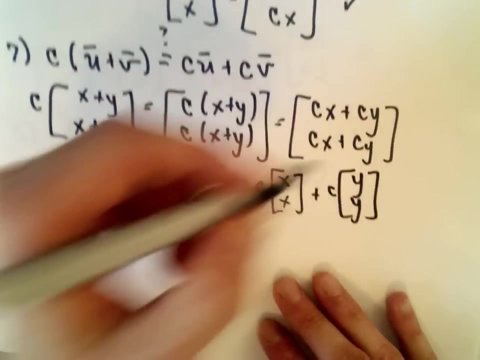 And again we can now break this apart- That's going to be cx, cx plus cy, cy. We can factor it back out. That's going to be c multiplied by xx plus c multiplied by yy, And that's going to be c multiplied by our vector u. 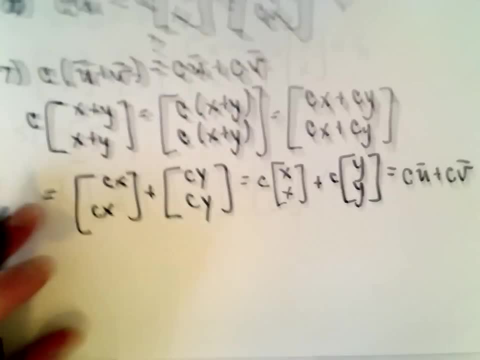 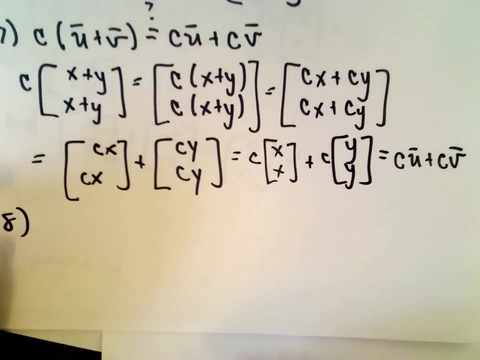 plus c multiplied by our vector v. So all right, Sorry if I'm going through this a little quickly. It's kind of a tedious problem and hopefully one that's not too terribly difficult. So let's see c plus d multiplied by u. 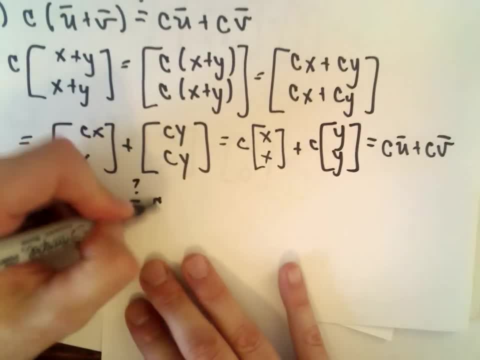 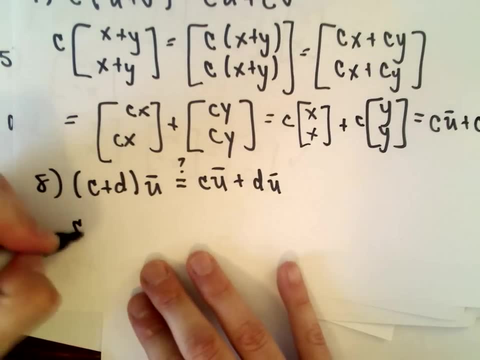 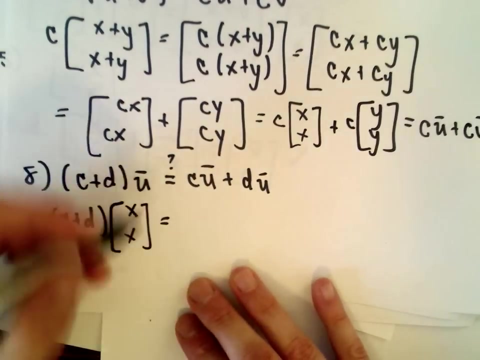 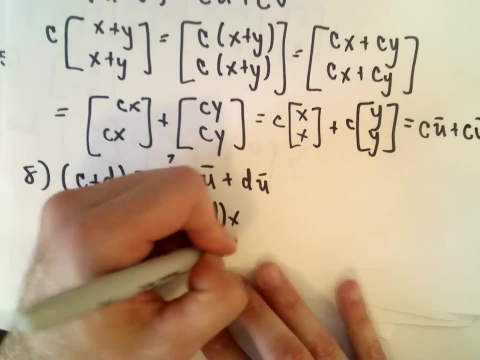 Does that equal c multiplied by u plus d multiplied by u? Well, let's see c plus d multiplied by u. That'll be x times x Or, excuse me, xx. So if we distribute, we would have c plus d multiplied by x.